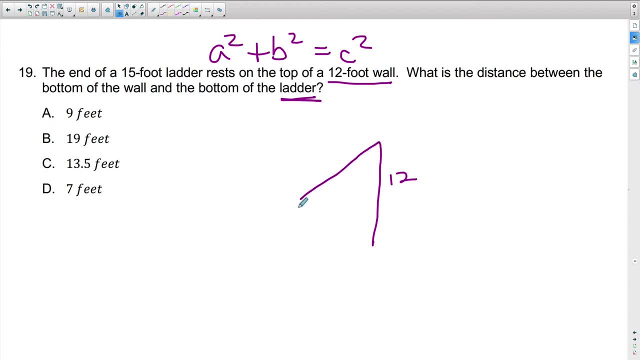 on top of the 12-foot wall And I'm going to have my ladder leaning up against the wall and it says it's 15 feet. What is the distance between the bottom of the wall and the bottom of the ladder? So that's going to be. 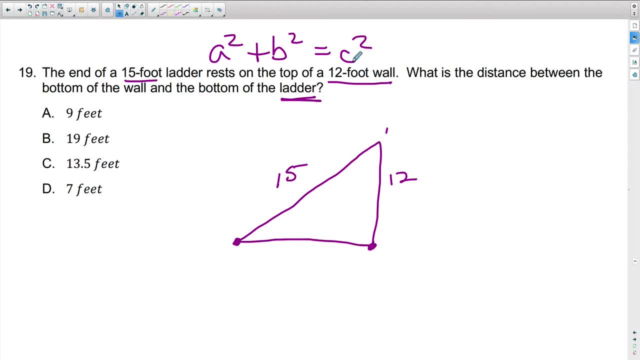 this side, right here. Now, when we're thinking about a squared plus b squared equals c squared, we want to make sure that we for c- we always use the hypotenuse- This is always c. Now a and b. 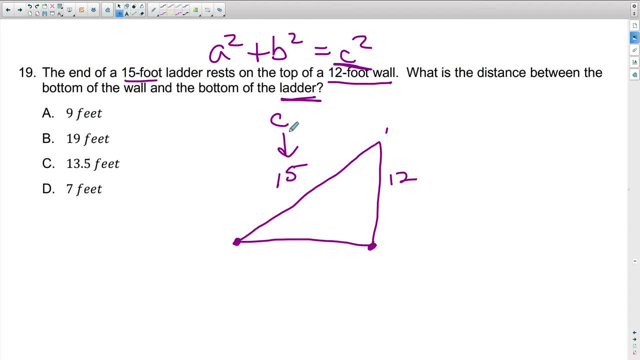 it doesn't matter, It can be either one of these legs, but the c has to be the hypotenuse or the longest leg of the triangle. So here we have two legs, We have a 12-foot wall and we have a 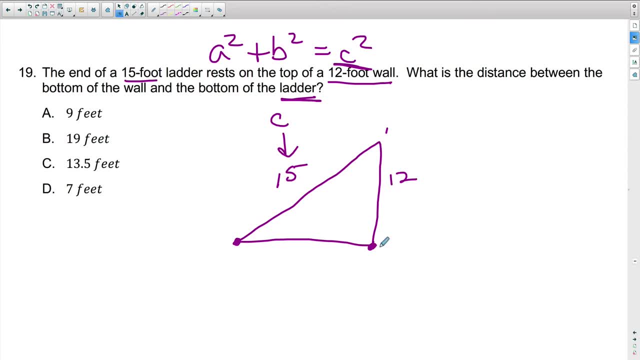 12,, 15, and we don't know the distance here. This is going to be our variable or our unknown. Let's go ahead and make that a, and let's make 12 our b. So if I'm going to put that in terms, 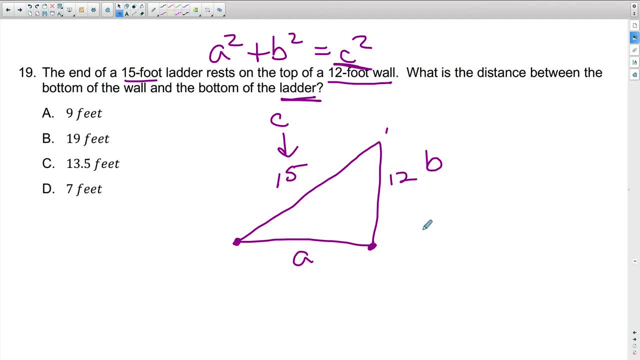 of the Pythagorean theorem. I'm going to have a squared which I don't know plus 12 squared equals 15 squared. Let's go ahead and figure these squares out. Well, a squared is always going to be a squared plus 144, which is 12 squared, which you can use your calculator. It's perfectly fine. 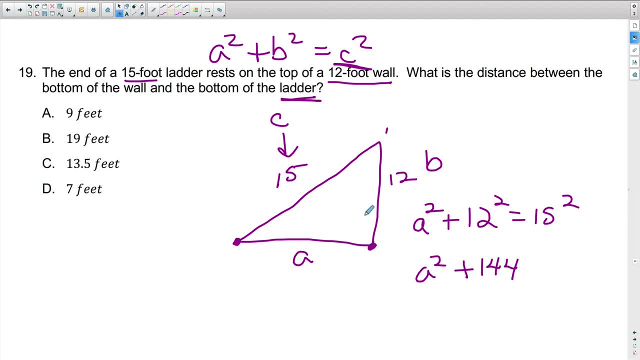 for you to use your calculator And let's do: equals 15 squared, which is 225.. In fact I had to use my calculator to do that, just to make sure. Now let's solve just like a normal algebraic equation. So if I'm solving like a normal algebraic equation, I want to go ahead and 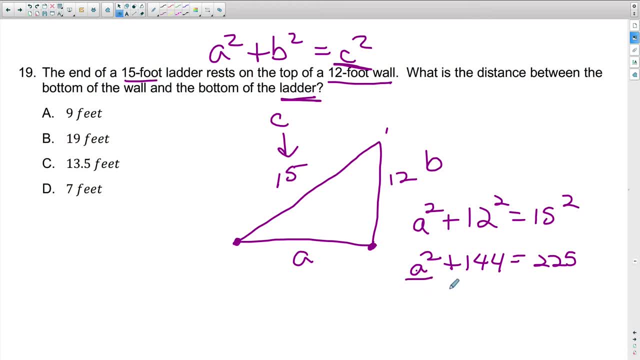 isolate my variables so I can solve for a. So what I want to do is subtract 144 from both sides. Remember, whatever I do to one side I have to do to the other. 5 minus 4 is 1.. 12 minus 4 is 8, and then this cancels out. So I have a squared equals 81.. 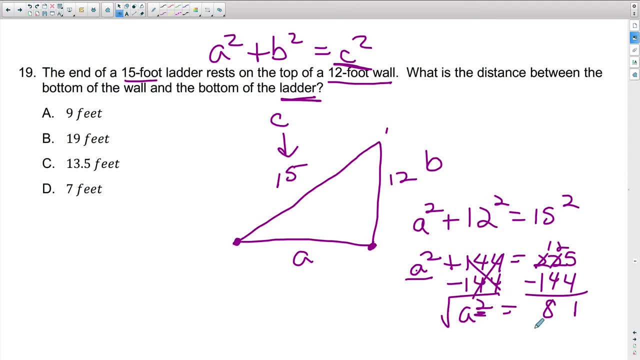 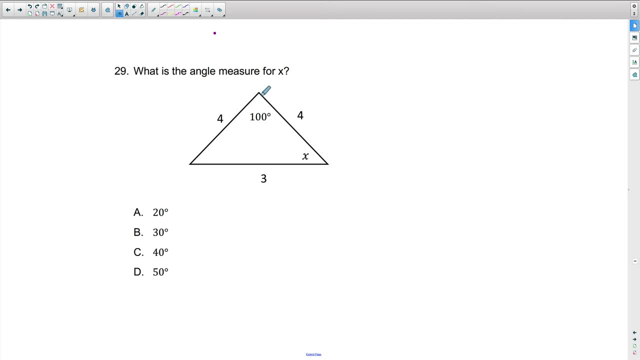 Then what I do to get rid of this squared. I basically take the square root of both sides, And when I do that I get a equals 9.. So our answer is a. Let's take a look at another way in which you'll have to deal with triangles on the GKT: the 6,, 12, and the 5, 9 math.